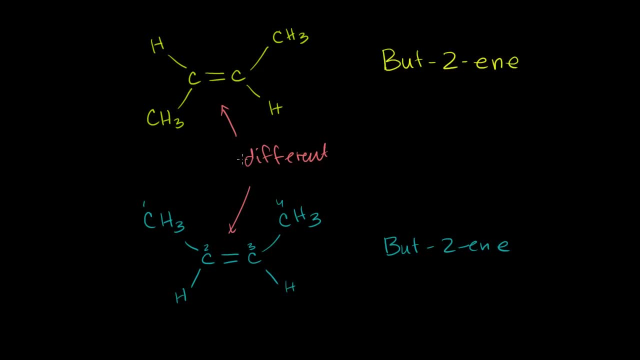 we have to have different names for them. Now there's two different naming conventions. One is kind of, I guess, the simpler naming convention And it works when we have one functional group on each of the carbons in the double bond. And then in the next few videos we'll 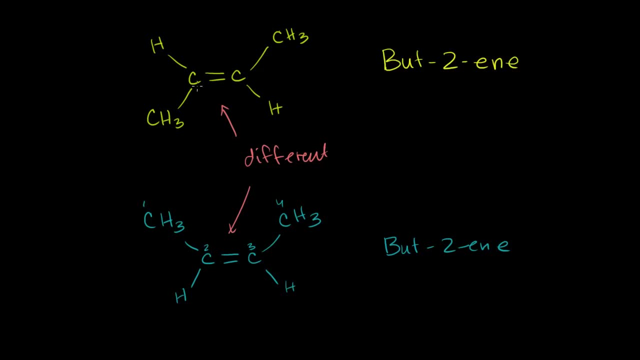 talk about the slightly more advanced naming scheme that will work when we have more than one functional group. So the first way to name it is if you have your functional group. So let me circle the functional group. So in this top one, our functional groups. 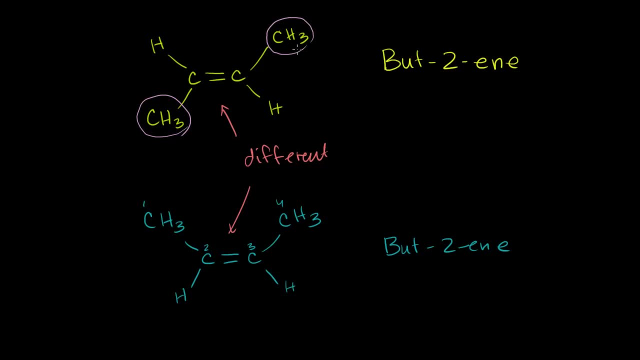 are on opposite sides, They're apart, They're on opposite sides of the carbon-carbon double bond. This is on the top, This is on the bottom. In this molecule, right here, our functional groups are on the same side. So when our functional groups are on different sides, 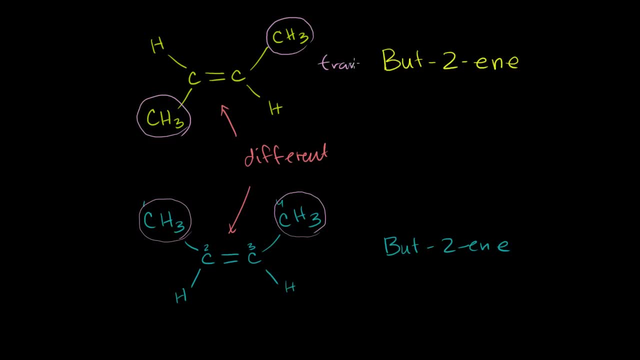 we could call it trans literally, for I believe, Latin for apart or Latin for opposite. I'm not a Latin scholar, so forgive me, But the functional groups are apart, so we call it transbutuene. The other convention to use comes from the germ. 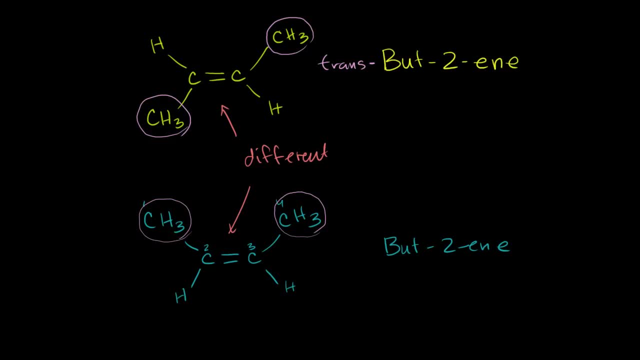 German for apart, And there we call it engagen. And instead of writing out engagen we write e in parentheses, So we would call them. Let me do this in different colors, since this molecule down here is blue, So we would call this ebutuene. 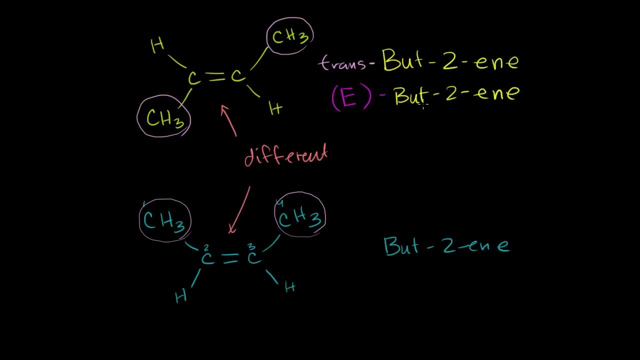 These mean the same thing, ebutuene, But this is now kind of the standard convention. We'll see this notation where you use engagen or e is actually more powerful. It can extend to when we have more than one functional group. 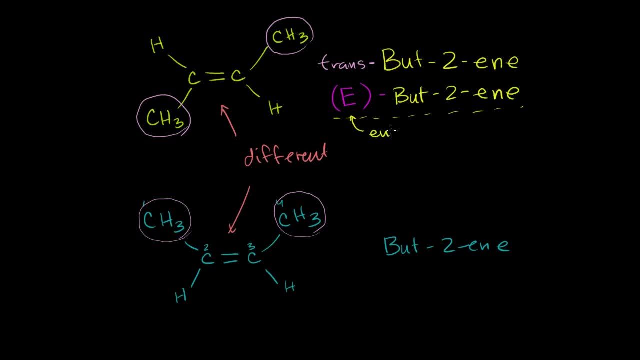 on each carbon. So let me just make it clear that the e stands for engagen, which is German for apart, Or at least I believe it is. I can't speak German, so I'll just have to take people's words for it. 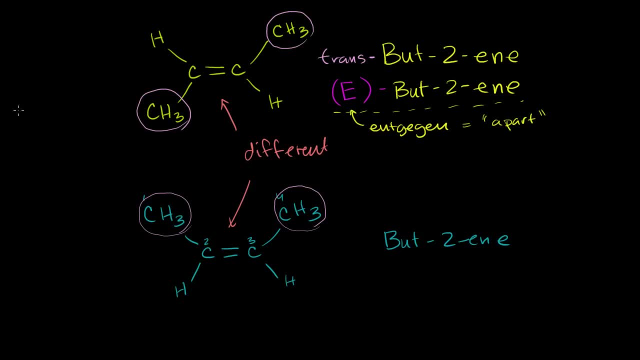 Now, in this situation where our functional groups are on the same side, you could call this cisbutuene- Cis, I believe, comes from the Latin for together, Or you could call it z, Or you could call it z-but-uene.